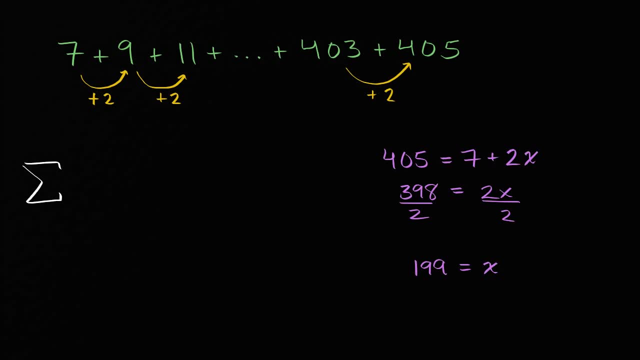 so there's a couple of ways we could think about it. We could think about how many times we've added 2.. So we could start with us adding to 0 times. the number 7 is when we haven't added 2 at all. 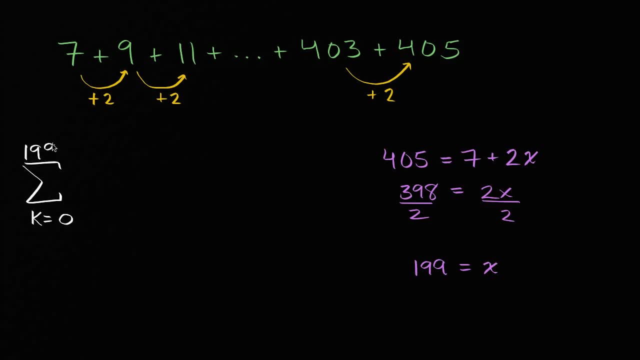 all the way to when we add to 199 times- And let's think about this a little bit- This is going to be- we could write it as: 7 plus 2 times k, 7 times 2,, 7 plus 2 times k. 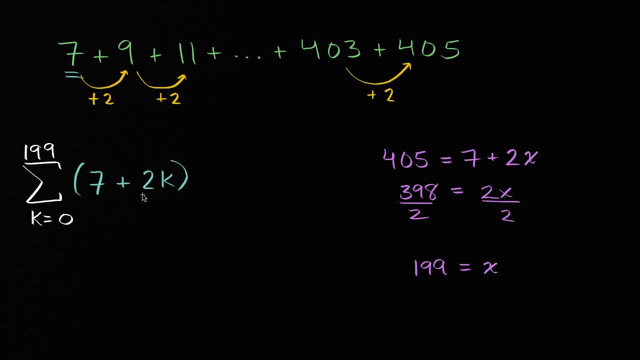 When k equals 0,, this is going to be 7.. When k equals 1, it's 7 plus 2 times 2.. Well, it's going to be 9.. When k is equal to 2, it's going to be 7 plus 2 times 2,. 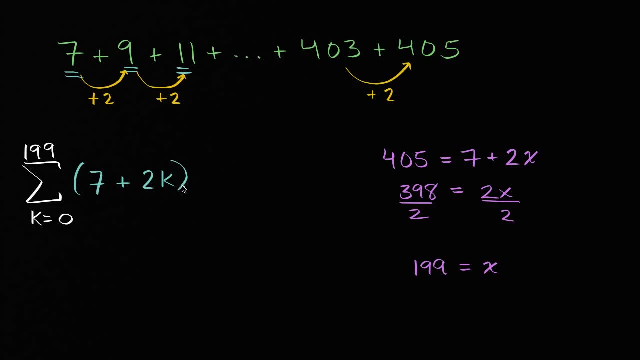 which is 11.. And all the way, when k is equal to 199,, it's going to be 7 plus 2 times 199,, which is 398,, which would be 405.. So that's one way that we could write it. 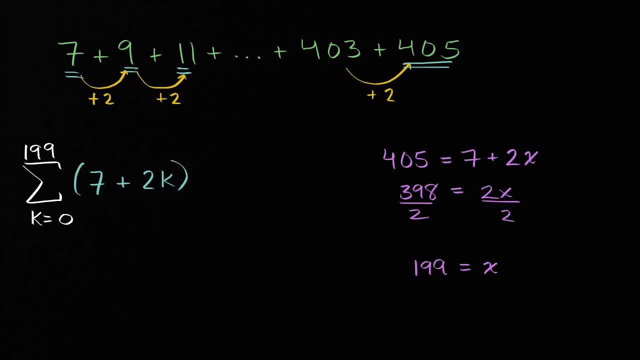 Another way. we could also write it as- let me just do this in a different color. We could, if we want to start our index at. k is equal to 1, then let's see it's going to be. the first term is going to be 7 plus 2 times k minus 1.. 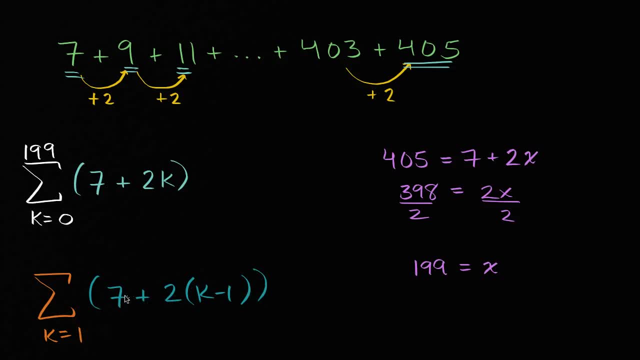 Times k minus 1.. Notice, the first term works out because we're not adding 2 at all. So 1 minus 1 is equal to 0. So you're just going to get 7.. Then, when k is equal to 2, the second term. 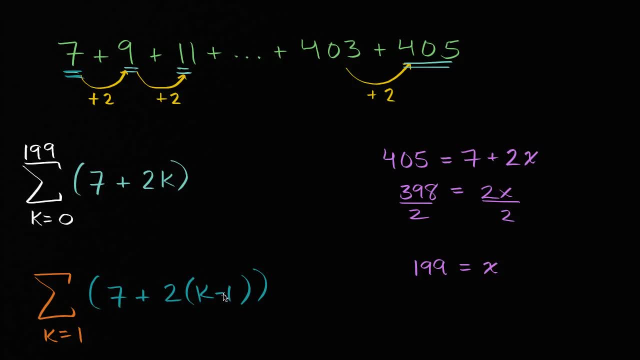 we're going to add 2 one time, because 2 minus 1 is 2.. So that gives us that one. And so how many total terms are we going to have here? Well, one way to think about it is: I just shifted the indices up by 1.. 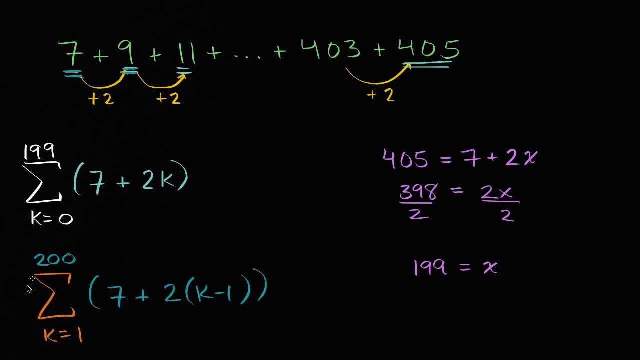 So we're going to go from k equals 1 to 200.. And you can verify this: When k is equal to 200, this is going to be 200 minus 1, which is 199.. 2 times 199 is 398,. 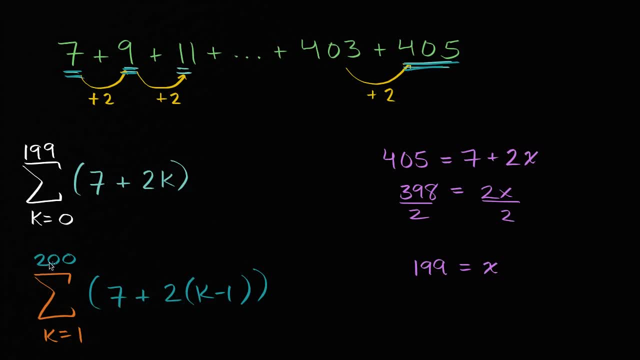 plus 7 is indeed 405.. So when k equals 200,, that is our last term here. So either way, these are legitimate ways of expressing this arithmetic series in using sigma notation.